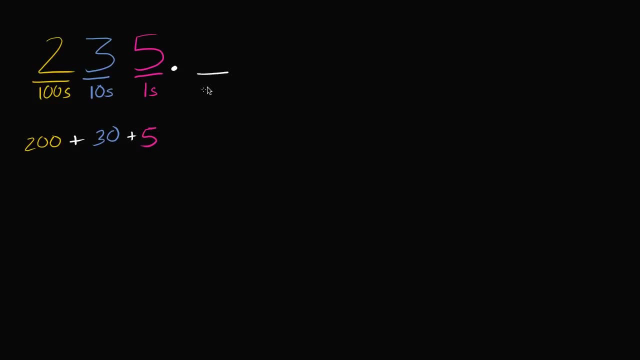 you are going to have find a new color. this is going to be the tenths place. This is going to be the tenths place. Well, what does that mean? Well, if, whatever number I write here, that tells us how many tenths we're dealing with. 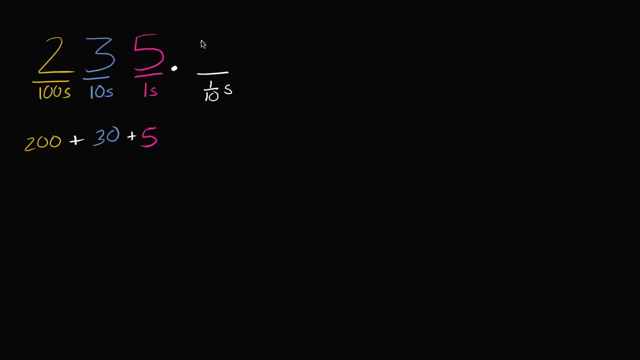 So if I were to write the number, if I were to write the number four right over here now, my number is two hundreds plus three tens plus five ones plus four tenths. So you could use this as four times one tenth, or you could write this as four tenths. 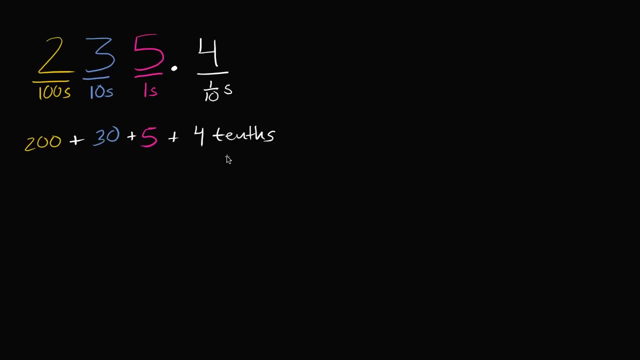 not tens. four tenths Or four tenths is the same thing as this right over here. So this is a super important idea. in mathematics I can now use our place values to represent fractions. so this right over here, this point four, this is four tenths. 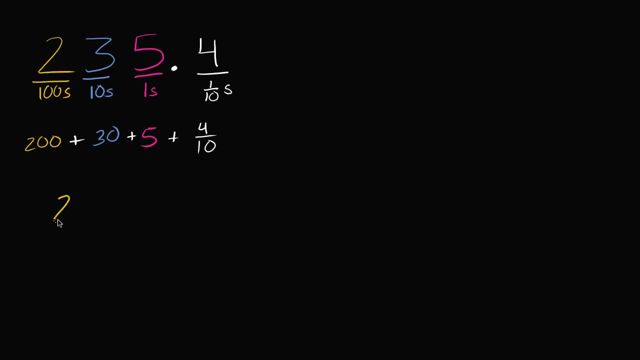 So another way to write this number. I could write it this way. I could write it as two hundred two hundred thirty. let me do the thirty in blue: two hundred and thirty, two hundred and thirty-five and four tenths. 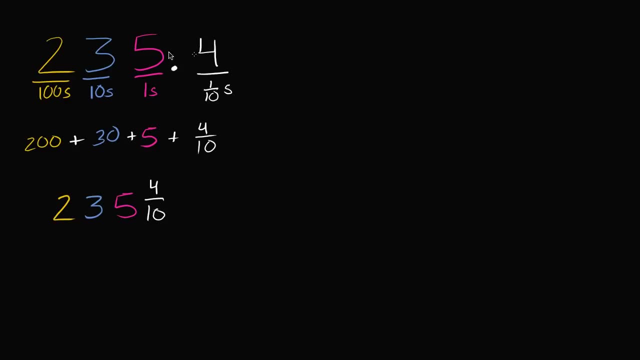 So I could write it like this as a mixed number. So this up here would be a decimal representation: two hundred thirty-five point four, and this right over here would be a mixed number representation: two hundred thirty-five and four tenths. 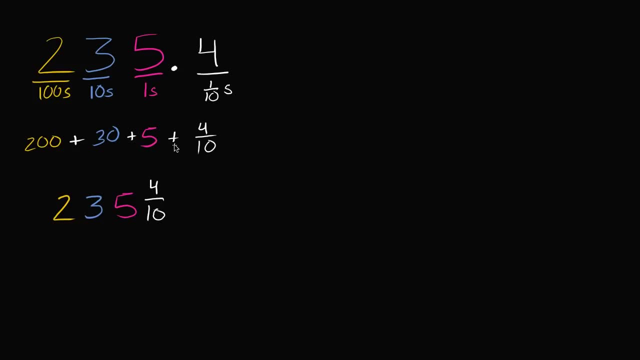 but they all represent two hundred plus thirty plus five plus four tenths. Let's look at a few more examples of this. So let's say I were to write the number. let's say I were to write the number zero, zero point seven. 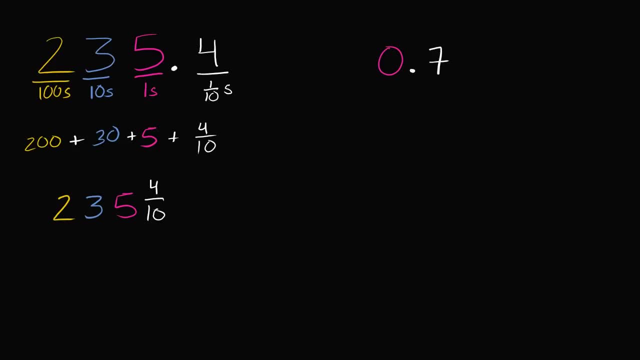 and actually let me go one space even further to the right. zero point seven, six. So what would this be If I were to write it as a fraction? So let's just think about the place value We have. our decimal point to the left of the decimal point is the ones place. 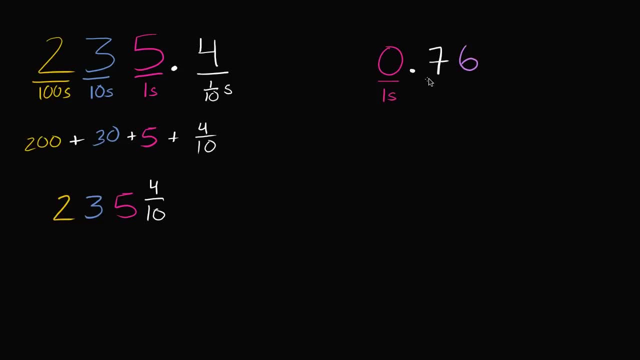 but I have a zero there, so this is zero ones. now I have seven tenths, so this is the tenths place and then this is going to be this place to the right of that. that's going to be. that's going to be. 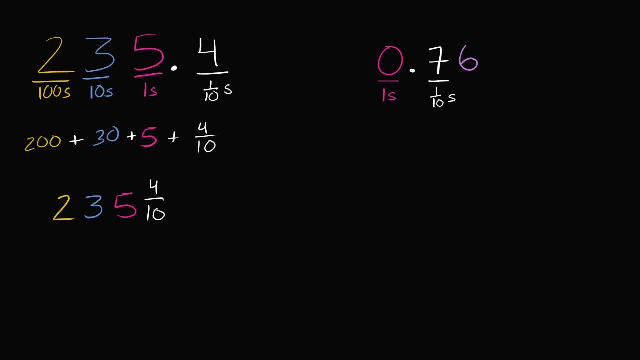 that's going to. we're going to divide by ten again, so this is going to be the hundredths place. So let me write this down: This base right over here is going to be the hundredths, the hundredths place. So this number right over here is: 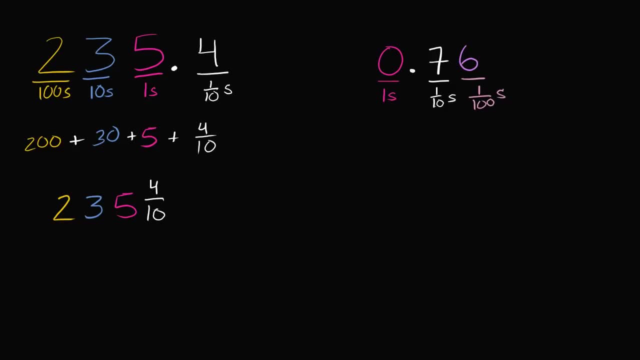 we can rewrite it as zero. let me write it this way: we could rewrite it as zero ones, zero ones plus seven tenths. plus seven tenths, not tens tenths. plus six hundredths plus six hundredths, not hundreds hundredths. 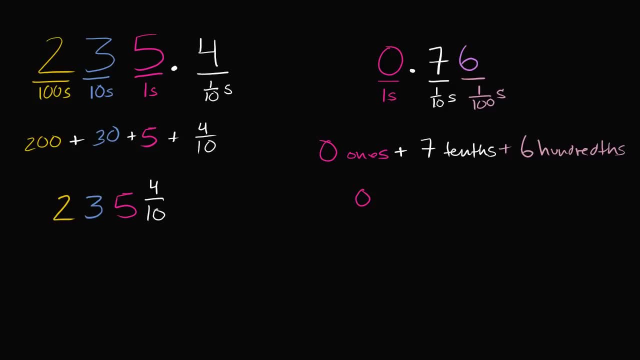 or we could write this as zero: plus plus seven tenths- let me write that a little bit neater: plus seven tenths plus six hundredths, plus six hundredths, six over one hundredths. So you could write this: seven tenths plus six hundredths. 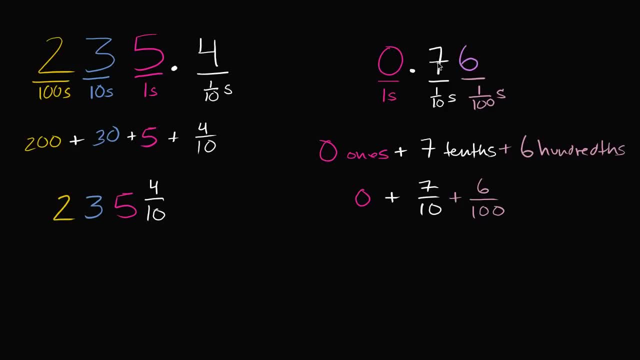 is exactly what this is. You could say: this is zero ones, seven tenths and six hundredths. Now, another way we could write this. you might be tempted. well, look, if we wanted to write it as a fraction or talk about it as a fraction. 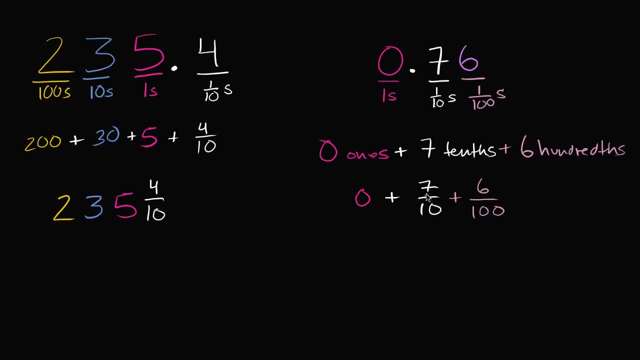 I could ignore the zero- that's not going to change the value of the sum- but I could add the seven tenths to the six hundredths. So how could I write seven tenths in terms of hundredths? Well, seven over 10 is the same thing as 70 over 100.. 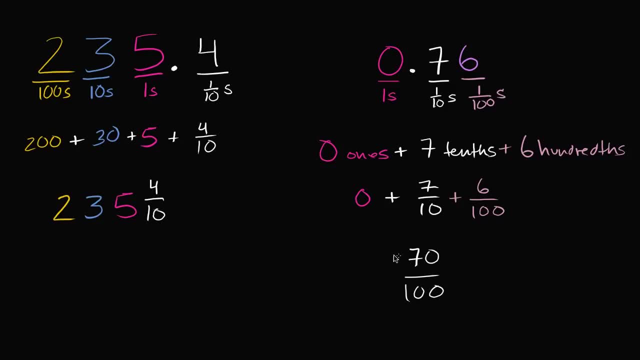 Is that seven tenths is the same thing as 70 over 100.. One way to think about it is: if I multiply the denominator by 10, well, I can multiply the numerator by 10 as well, but that will not change the value of it. 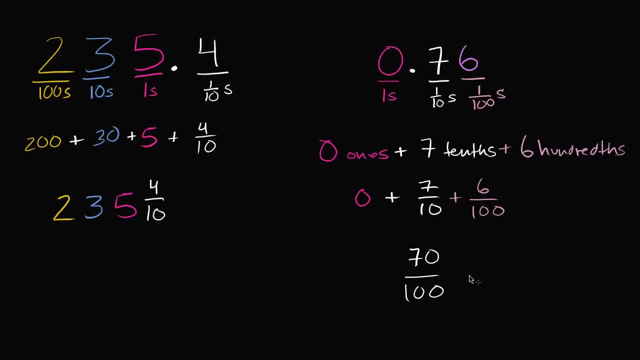 Seven tenths is the same thing as 70 hundredths, and then you could add six hundredths to that, six hundredths to that, and what will that give you? Well, that's going to give you 76 hundredths, Seventy six hundredths. 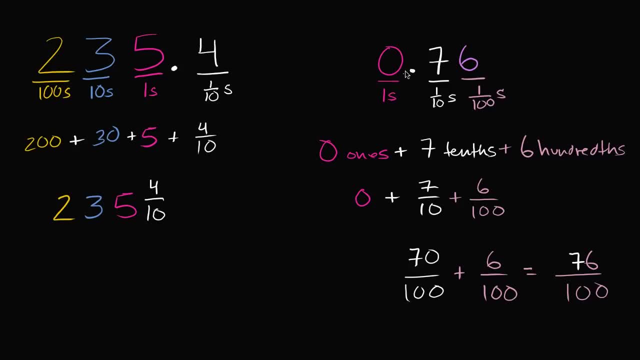 So this number up here, a lot of people will call this. they might say zero point seven six or they might call this 76 hundredths, Seventy six hundredths. This is the hundredths place. this is the tenths place.